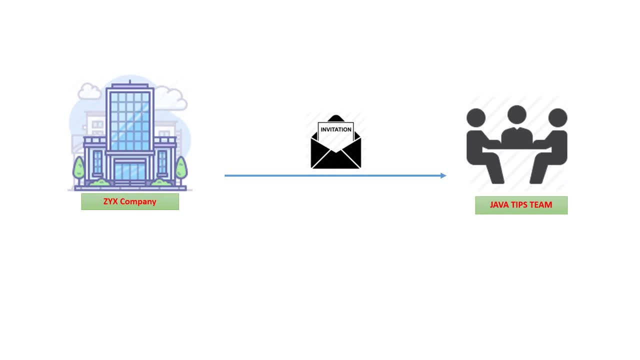 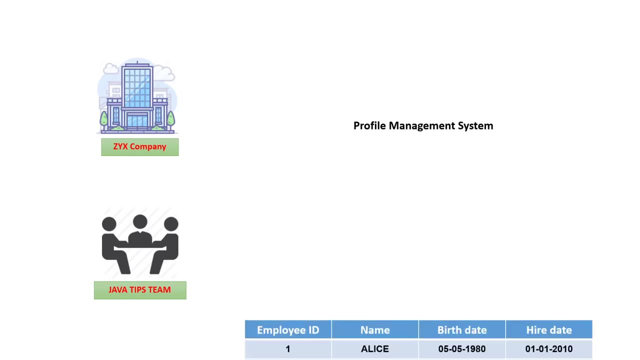 Send us an invitation to our Java tips team Next day. Zix company asked us to build a profile management system. This profile management system enables their employees to browse their own data like employee ID name, birth date and hire date. It's pretty simple. 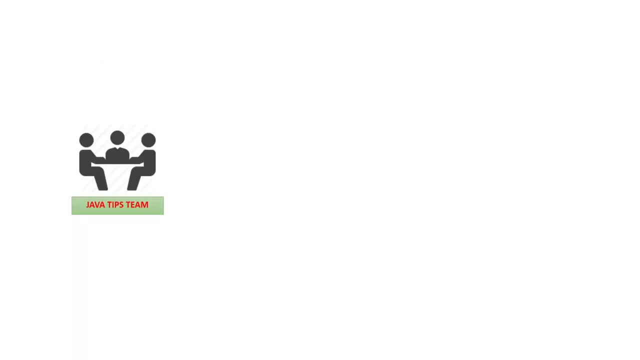 Next day, our development team held a meeting and the business analyst said that Zix company already has HR systems And this is what Zix company wants. This HR system works on the database and this database contains all the data we need to fulfill our project management system. 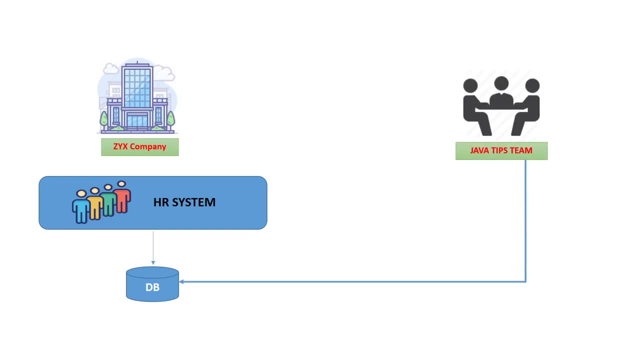 Okay. On the next day our development team tried to contact with HR system team and asked them to give us direct access to the specific table which gives us the data we need, And HR system team approved. One week later the system was ready. 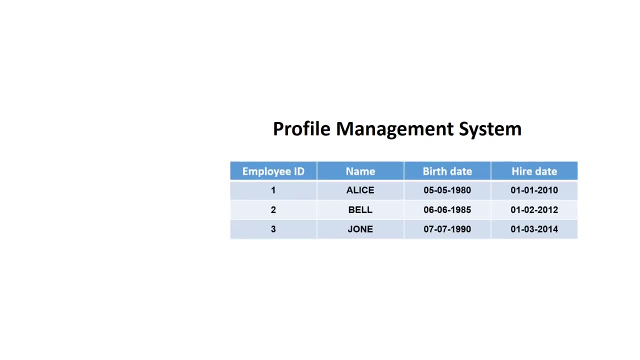 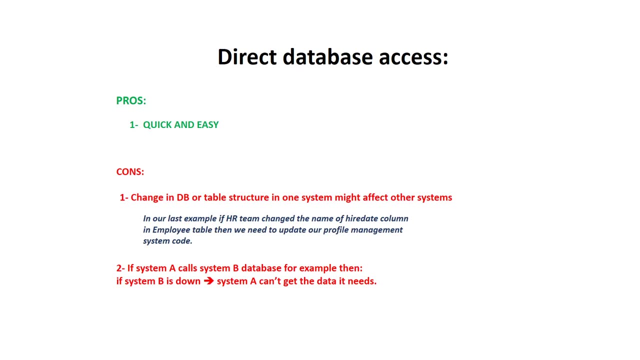 And the client was happy. Now let's have a look on the pros or advantages, and the cons or disadvantages of using direct database access to establish system integration. Two months later, HR system was ready And the client was happy. Now let's have a look on the pros and the cons of using direct database access to establish system integration. 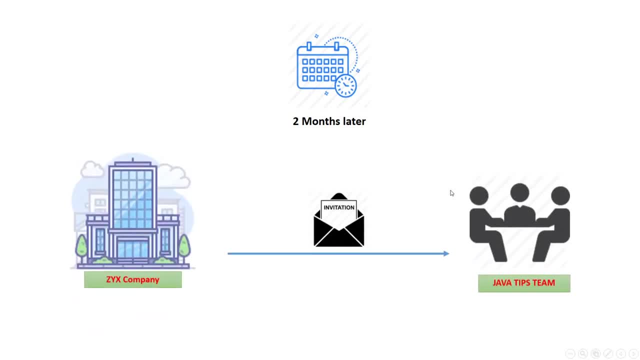 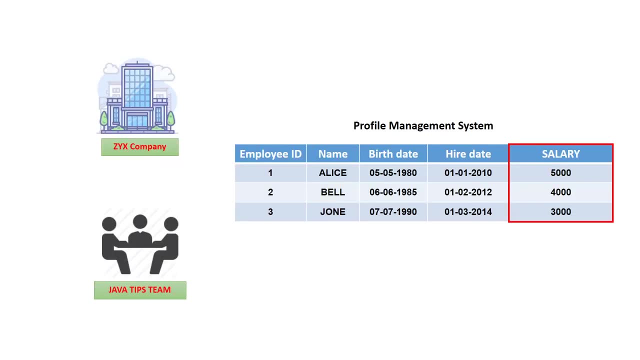 Two months later, we received an invitation from this company to hold a meeting. On the meeting, this company said that the application we already provide is good, but now they want their employees to be able to see their salary on the profile management system. 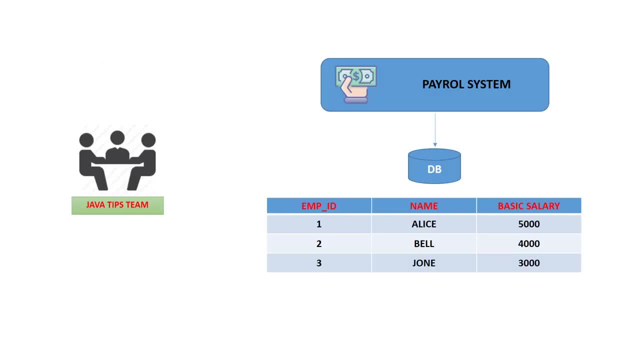 Okay, it's all so easy. Next day, our development team held a meeting again and the business analyst said that this company also has a payroll system which contains the basic salary which we need to display in the new version of the profile management system. 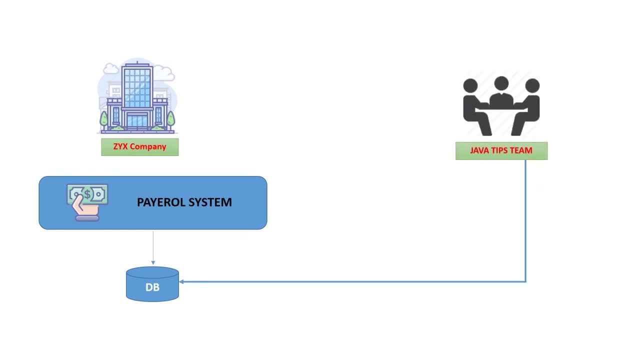 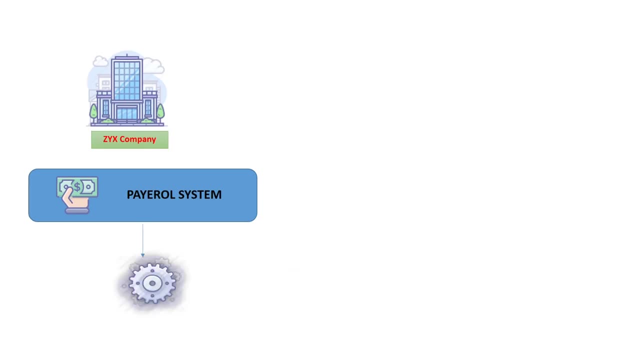 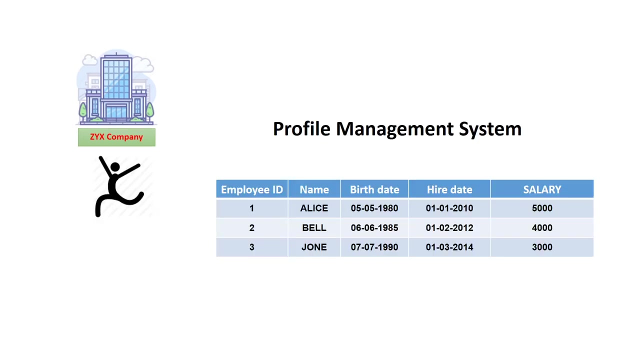 Next day our development team tried to get access to the payroll system database, but they refused. Okay, But they said that they can give us web services so we can consume the salary we need. This was okay. One week later, we also was able to modify the profile management system and add the. 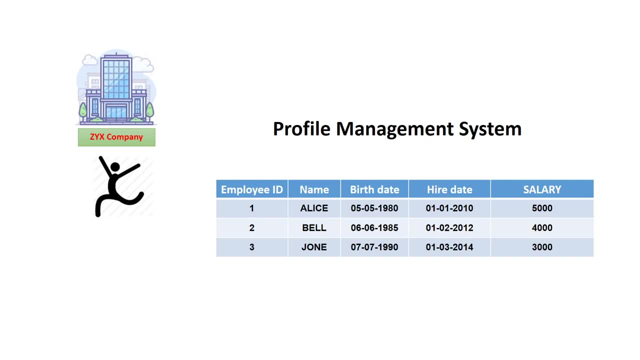 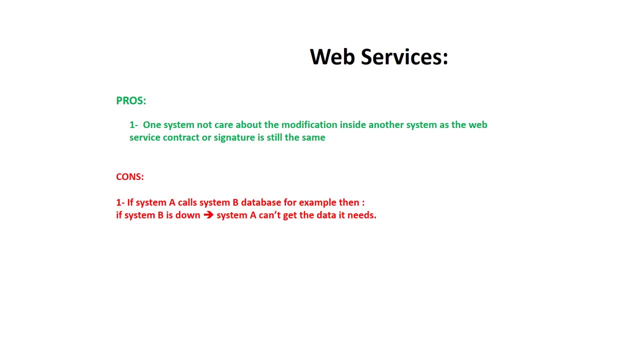 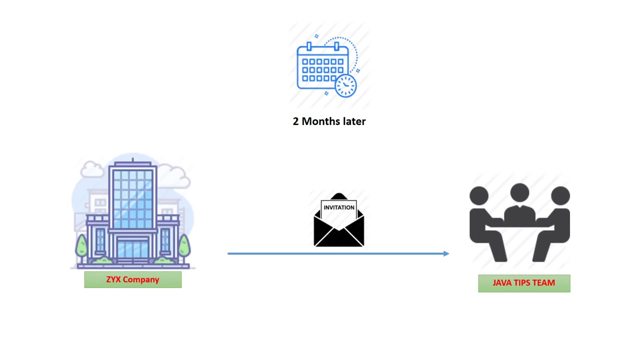 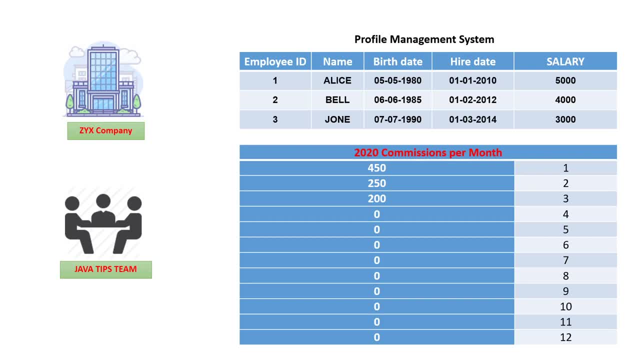 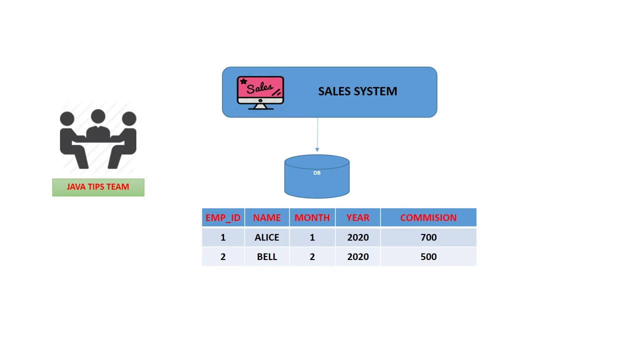 now After several years. they said they think it's okay now. but sales employee inside this company wants to see their monthly commission on their profile, for example in January, on February and so on. okay, next day when we hold a meeting. business analyst said that this company already 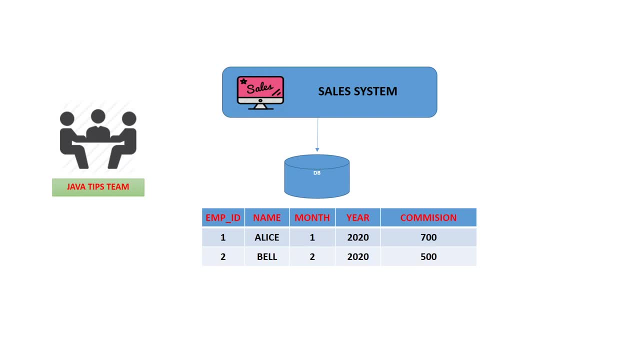 has a sales system and this system work with database which contains a commission we need to display in the profile measurement system. business analyst said that this sales system team cannot give access to their database directly, but they can give us a web services and in this web services we can. 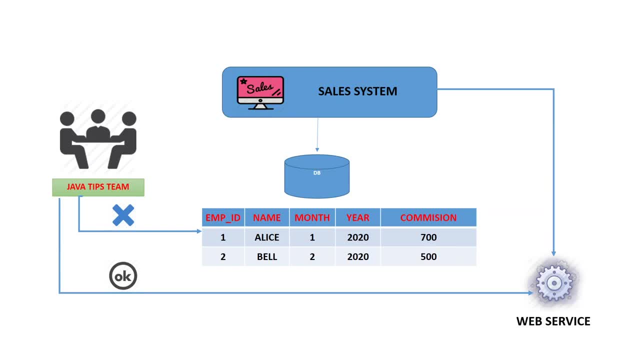 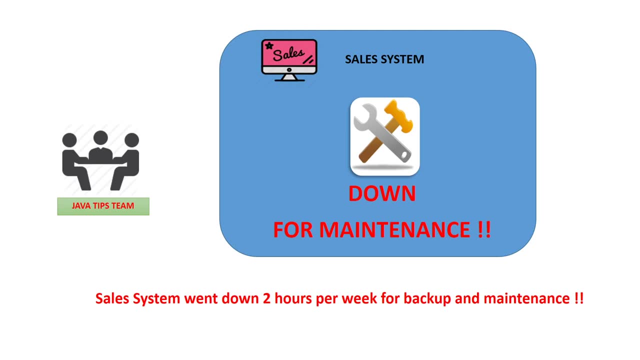 consume it to get the commission per employee per month. but there was a problem with sales system. that it's when there is a problem with their system, that it's when down two hours per week for pickup and maintenance and that was unacceptable for the six company. what is the solution?